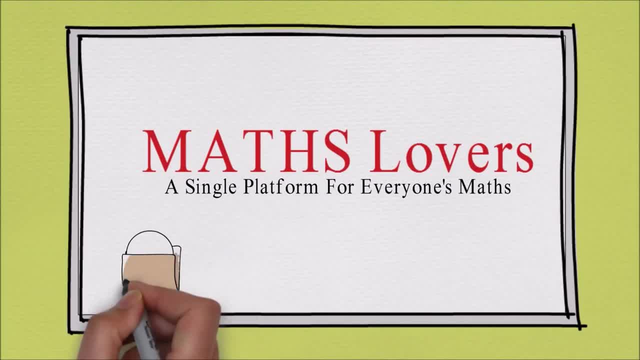 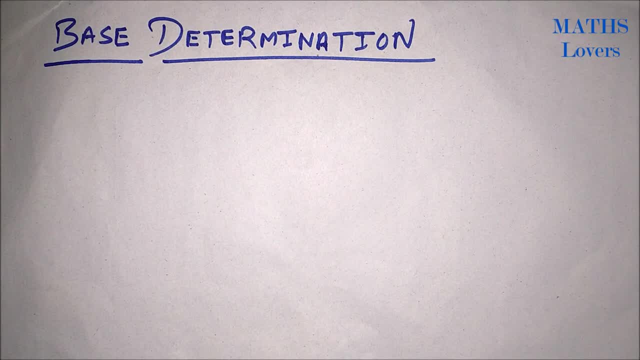 Hello math lovers. In this video we will understand base determination. Base determination is one of the important topic for aptitude preparation In general. all the addition and subtraction we are familiar with have base 10.. Let's take a example, for it Like: 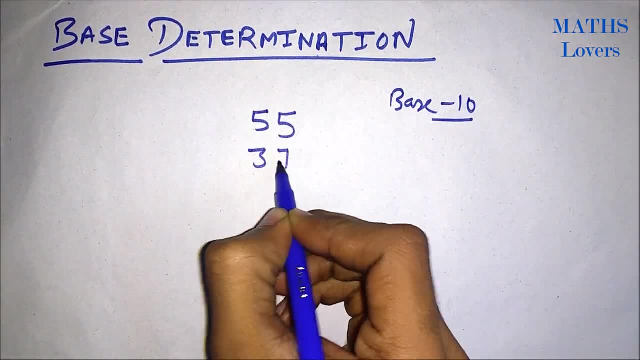 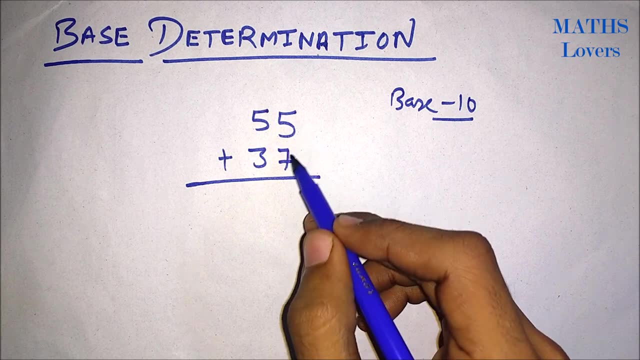 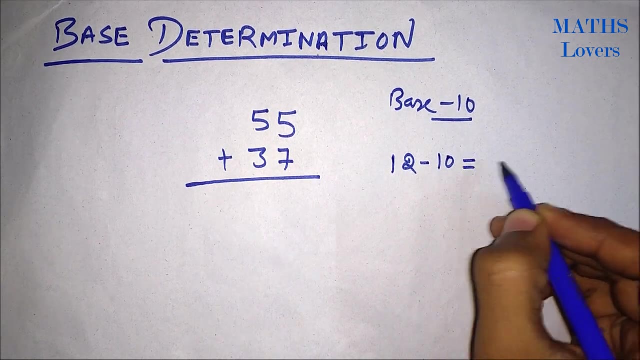 if we want to add 55 and 37, then how we will do. We know that 5 plus 7 is equal to 12. So we will write 12. Then base is our 10. Then we will subtract it from 10.. Then how? 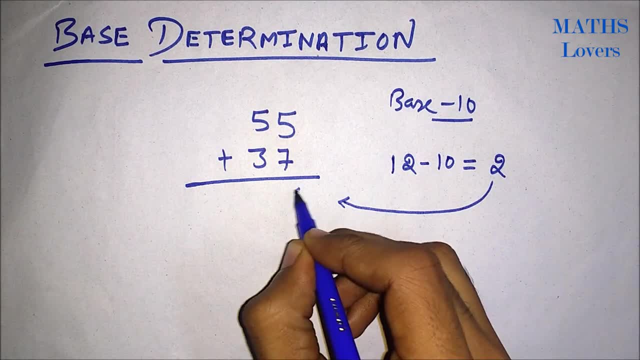 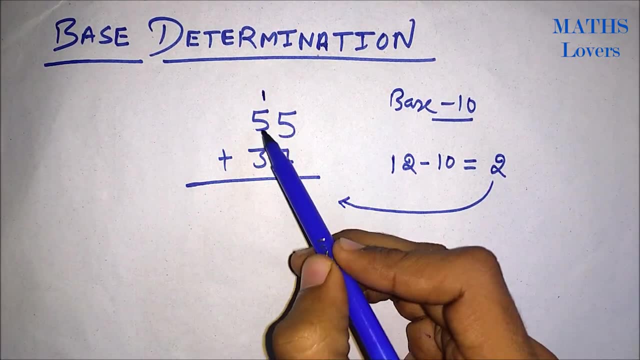 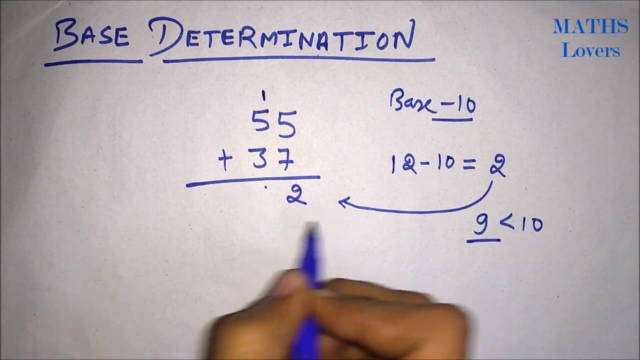 much, we will get 2.. We will write 2 here, And we have subtracted 10.. Then we will carry forward 1.. So now we will add 5 plus 3 plus 1. That is equal to 9.. 9 is less than 10.. That's why we will write it as it is. So what if? 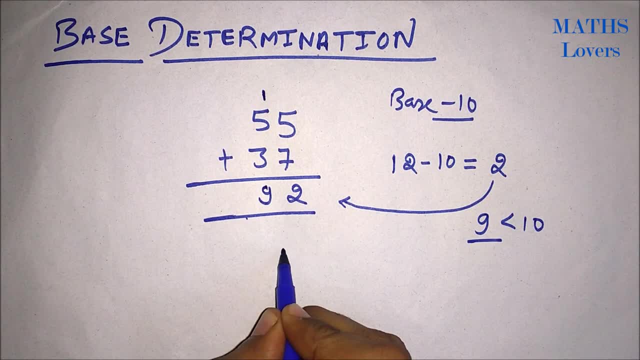 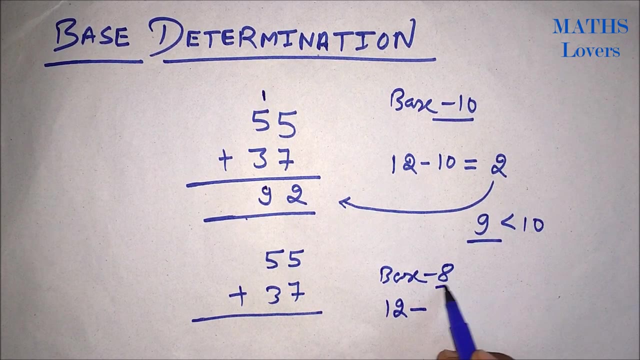 I change the base 8?. So let's see 55 and 37 plus Now our base is 8.. So if 5 plus 7, it is again 12.. Then now I have to subtract it from 8. Because our base is 8. Then we 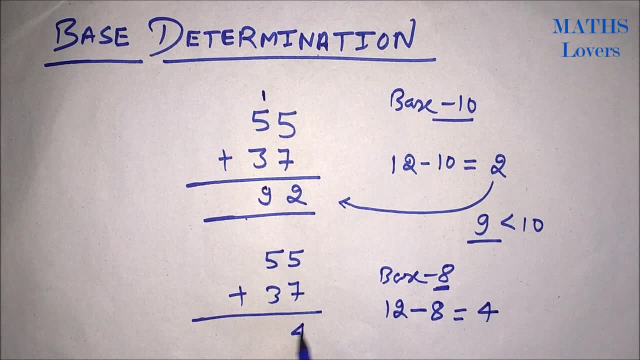 get 4.. So I will write 4 here, And I have subtracted 8 one times. That's why I will write: carry forward 1.. Again, I will add 5 plus 3 plus 1. That is equal to 9. Again. 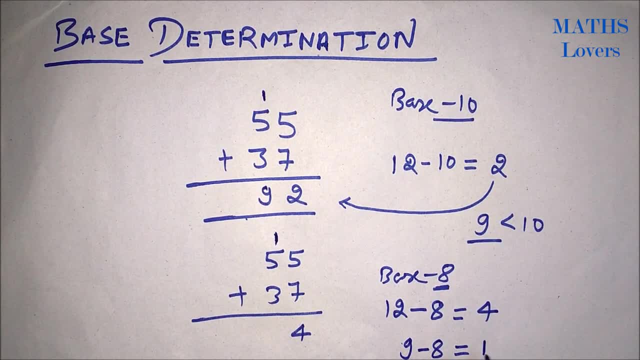 I will subtract 9 minus 8. That is equal to 1. So I will write 1 here and carry forward 1.. That is 1 as it is. So our summation will be 114 when base is 8.. Let's see some more. 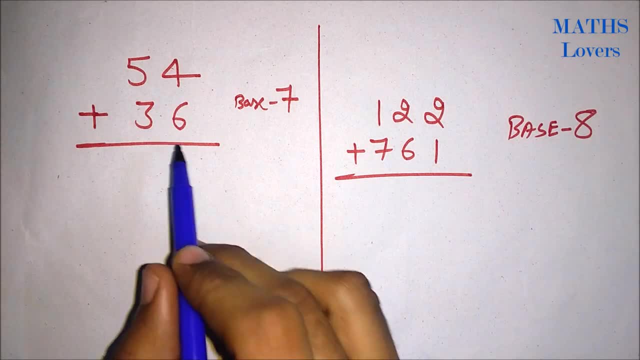 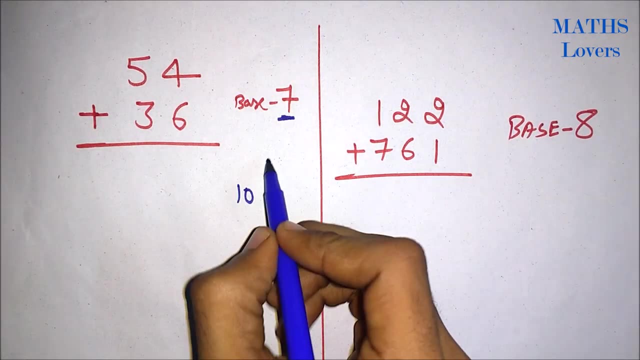 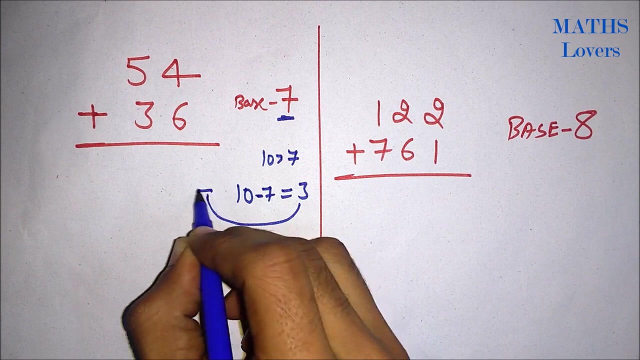 examples Here: 54 plus 36 and base is 7.. So 4 plus 6 is 10.. Again, we have to subtract. 10 is greater than 7.. That's why we have to subtract it from 7.. So we will get 3.. So here we will. 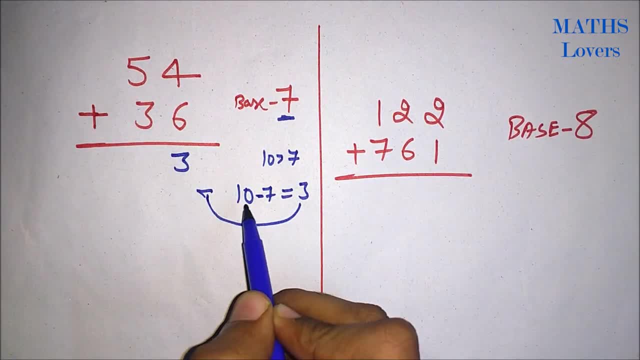 write 3.. Then 1 will be the carry forward, because we are subtracting 7 one times. That's why 1 will be carry forward. And now 1 plus 5 is 6.. 6 plus 3 is 9.. Again, 9 is greater. 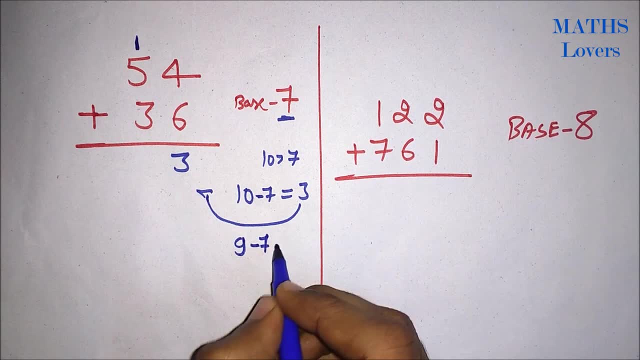 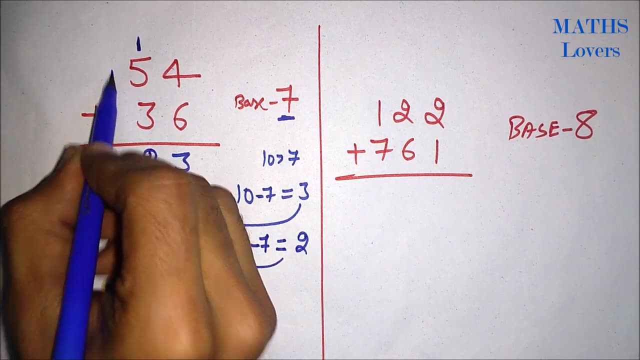 than 7.. That's why we will subtract it from 7.. So we will get 2.. That's why here we will write 2. And 1 will be the carry forward. So here no number is there. That's why we will write. 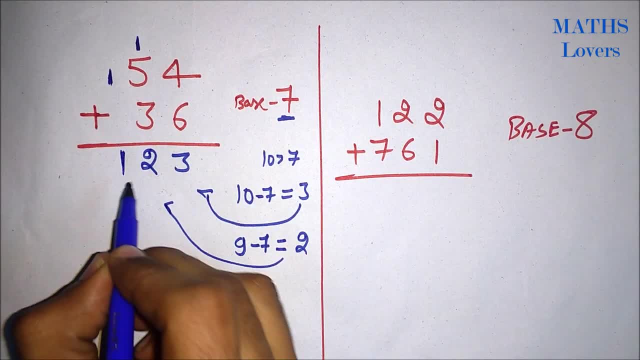 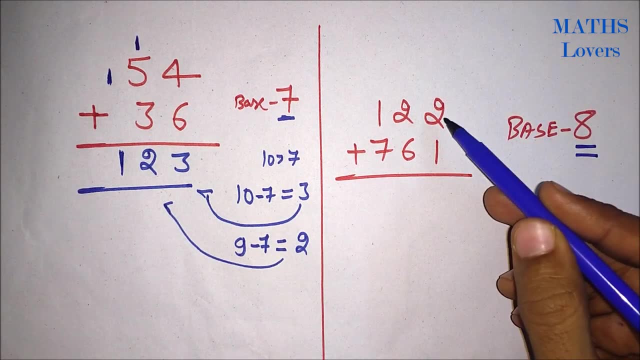 1 as it is, Because 1 is less than 7, that's why we will write 1.. Let's take another example Here. base is 8. So 2 plus 1 is 3. And 3 is less than 8.. That's why we will write it as: 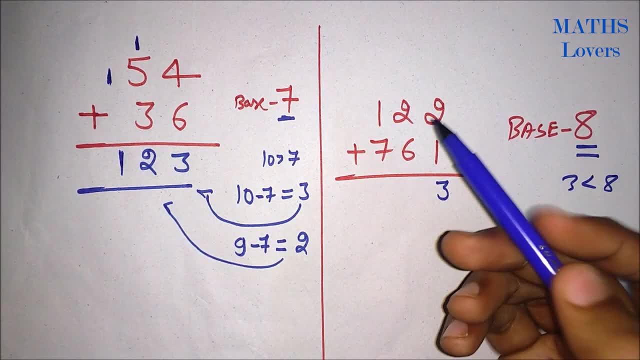 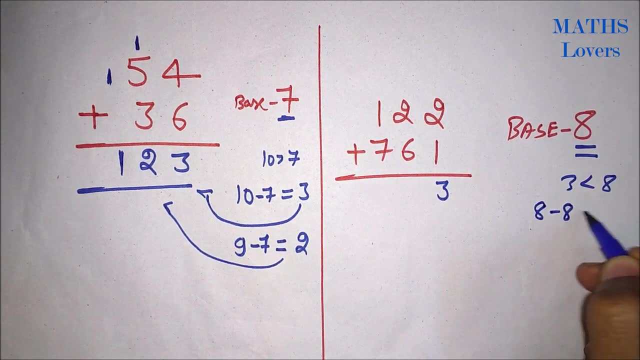 it is. So we have no subtracted 8. that's why there will be no carry forward Now. 6 plus 2 is 8 and 8 is equal to 8. that's why 8 minus 8 equal to 0.. 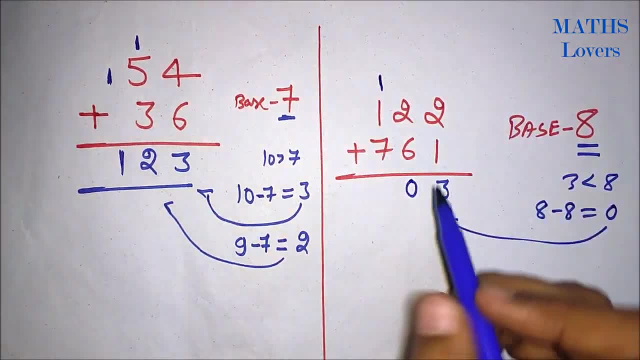 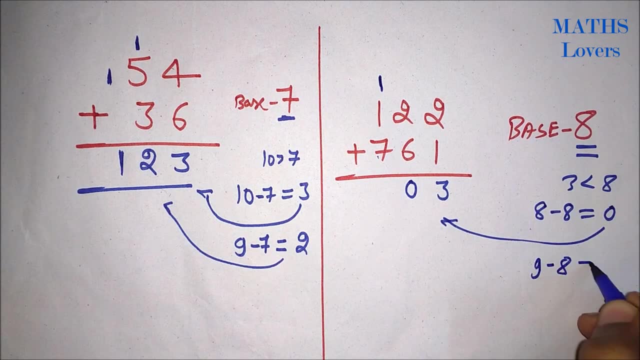 So here we will write 0, and 1 will be the carry forward. So now 1 plus 1, 2 and 7, 9, 9 is again greater than 8. that's why we will subtract it from 8 and we will get 1.. 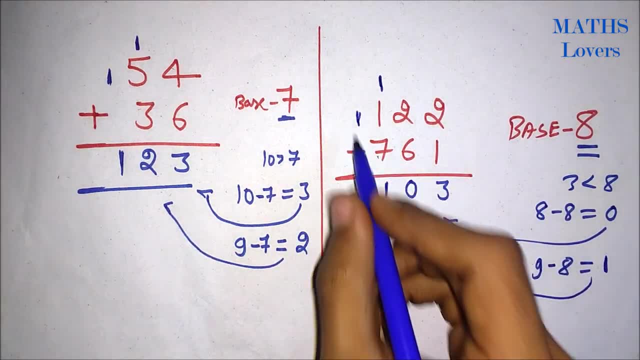 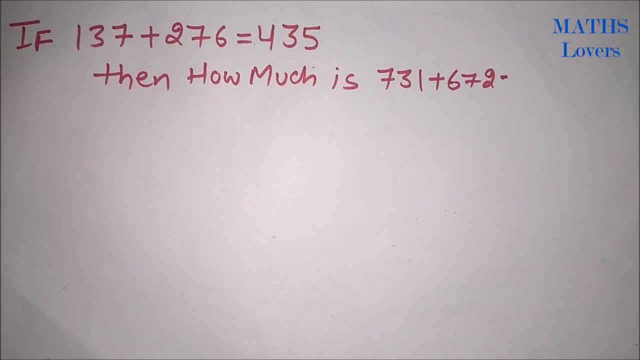 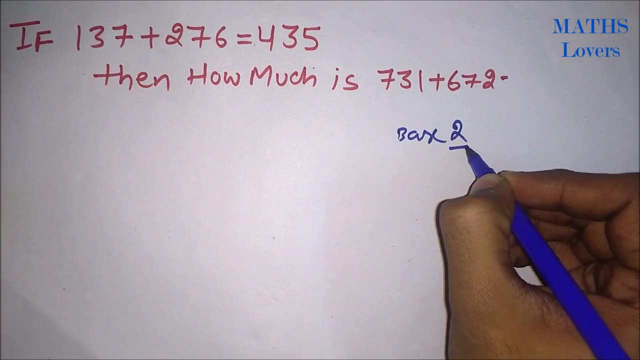 So here again we will write 1 and 1 will be the carry forward, So 1 will be as it is. So our summation is 1 1 0, 3.. Let's hold a question on it. Before that, I would like to tell you one thing: that if base is 2, or we call it binary- 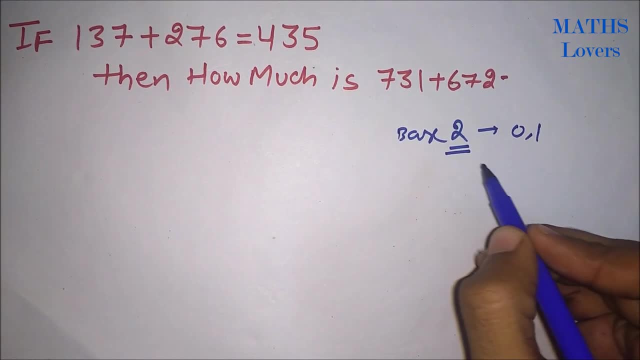 If base is 2, then digit can be 0 and 1.. If base is 3, then digit can be 0, 1, 2.. Like this, if base is 8, digit can be from 0 to 7, like 0, 1, 2, 3, 4, 5, 6 and 7.. 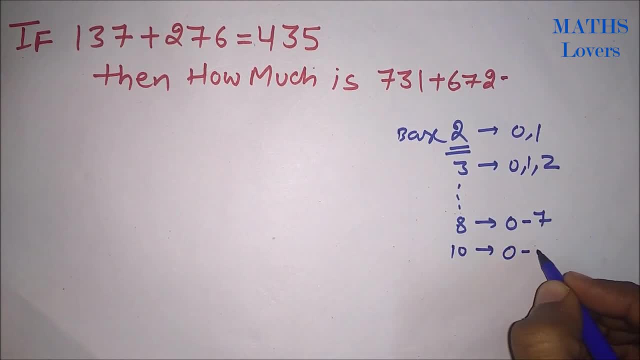 Like this: if base is 8, digit can be from 0 to 7, like 0, 1, 2, 3, 4, 5, 6 and 7.. And if base is 10, then digit can be 0 to 9.. 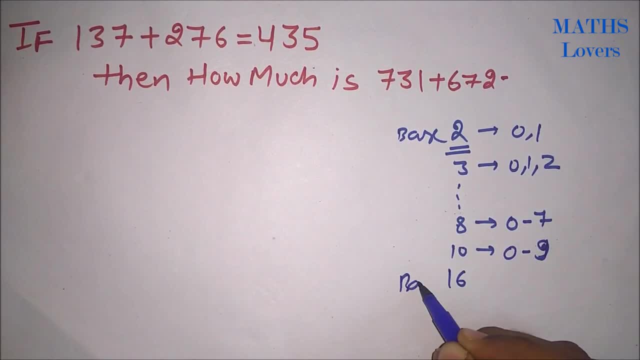 Similarly, if anyone says: if base is 16, then what can be digit? Digit can be up to 15.. For writing 10, we use a. For writing 11, we use b. Like this for 12 c, 13 d, 14 e and 15 and 15 f. 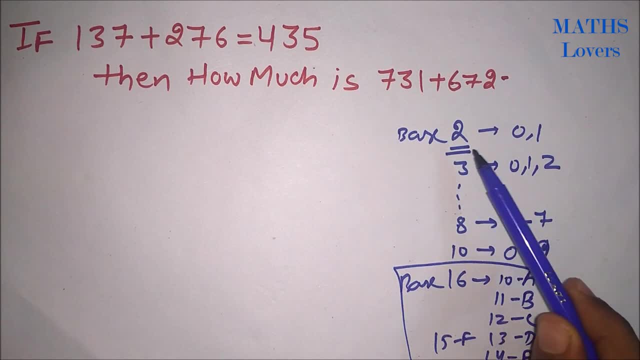 So always remember that if base is 10, then digit can be from 0 to 9.. Similarly, if anyone says: if base is 16, then what can be digit? Digit can be up to 15.. For writing 12, we use a. Like this for 12 c, 13 d, 14 e and 15 f. So always remember that if base is 10, then digit can be from 0 to 9.. So always remember that if base is 10, then what can be digit? 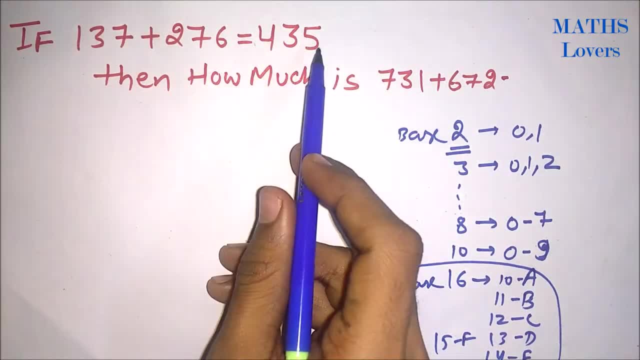 Digit can be up to 15.. So always remember that if base is 2, then digit can be from 0 to 9.. So in this question we can see that 137 plus 276 equals 435, so maximum number- maximum digit is biggest- is 7.. 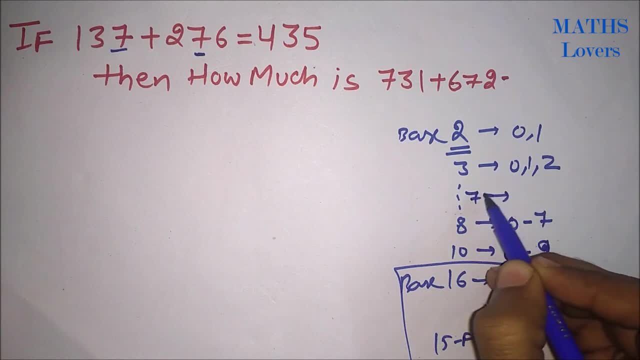 That's why base can not be 7, because in base 7 digit can be only 0 to 6, but here digit 7 is also there. That's why base will be greater than 7 means 8, 9, 10 and all. 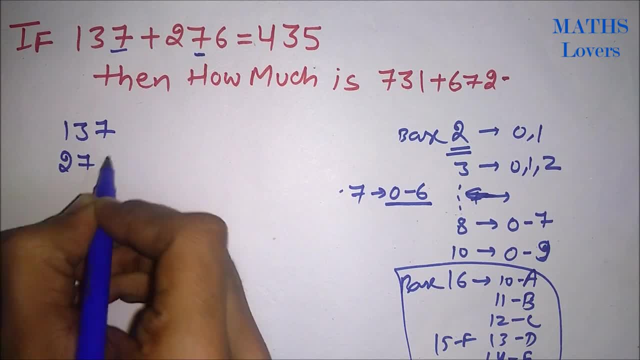 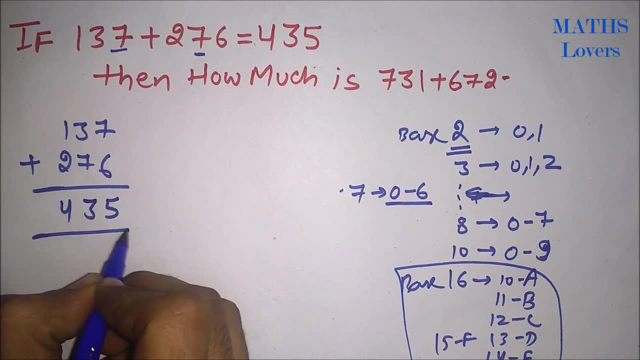 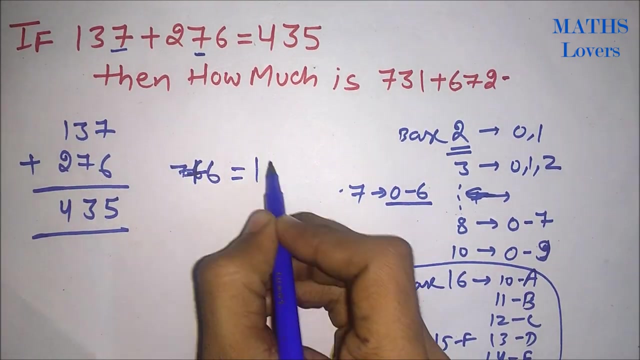 for this question we have to determine first the base. so so 137 plus 276, that is equal to 435. now, here we can see that 7 plus 6, 7 plus 6, will be 7 plus 6 will be 13. that's why- and here it is coming- that 5, so we are writing 5. so if i 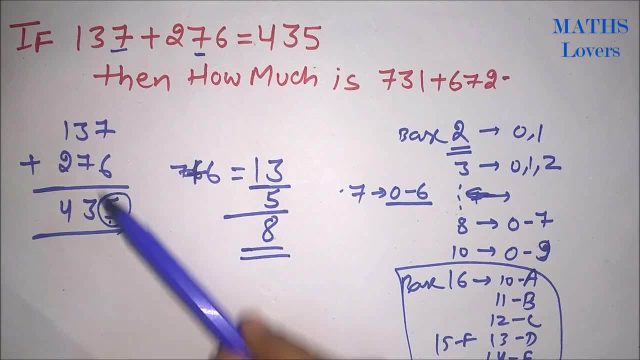 subtract 5 it here, i am getting 8. that means 7 plus 6 plus 13, and if i subtracting 8 from that, then i am getting 5. that's why our base will be 8.. so now let's solve this. 736 and 672: we have. 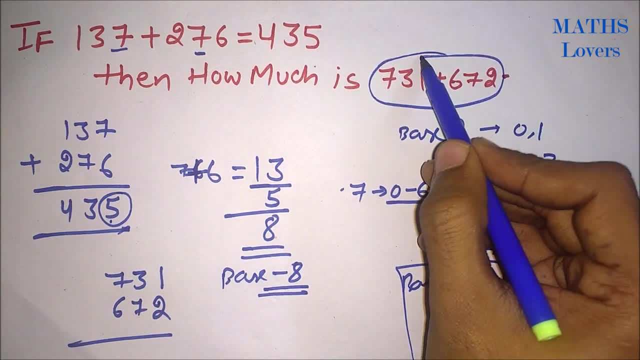 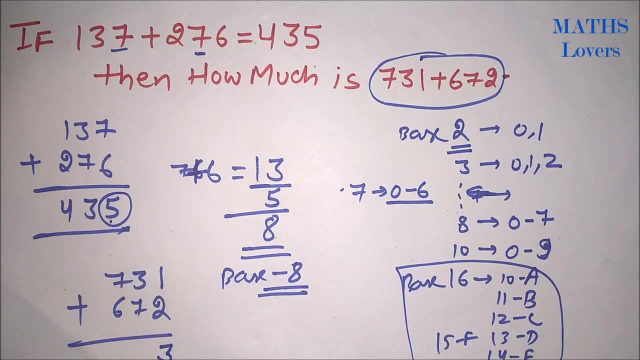 got the base equal to 8. that's why we have to solve this problem same as with base 8. so 1 plus 2 is 3. it is less than 8. that's why we will write same at as it is. then 7 plus 3 is 10, so we have to subtract it from 8. that's where we got. 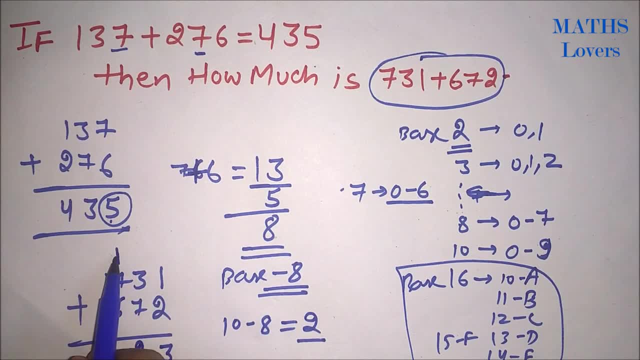 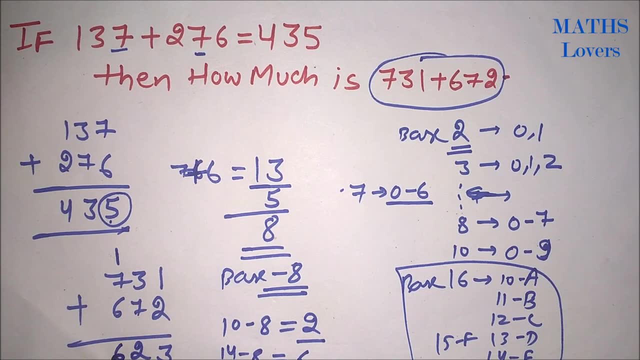 2. so here i will write 2, 1 will be carry forward. 7 plus 1, that is 8 plus 6, 14. if i subtract 14 from 8, that i get 6. that's why i will write 6 here, and 1 will be carry forward and 1 as it is. 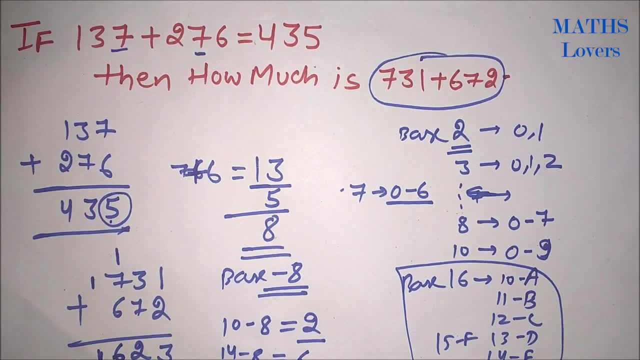 so our answer is 1, 6, 2, 3. so this is what does the addition. so, like this, we can add one more thing: i would like to tell that if you want to solve this problem, then you have to write 7 plus 3 as it is.